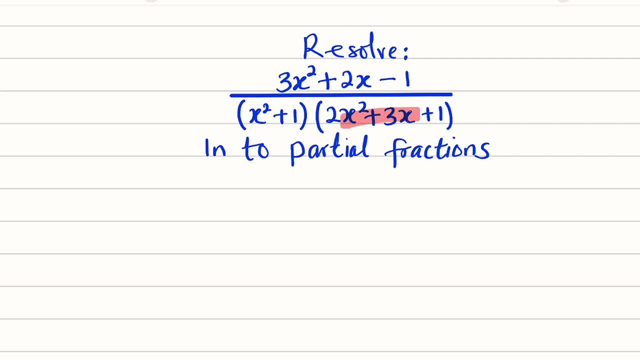 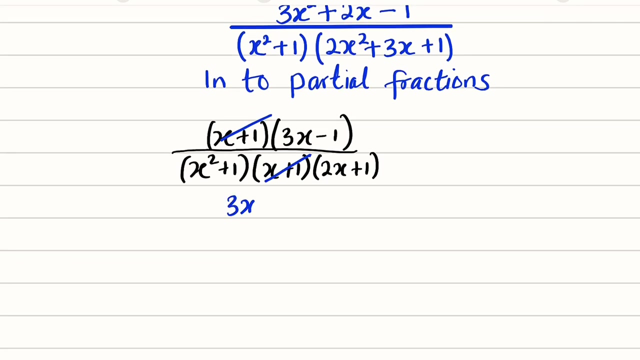 But considering these two factors, this is reducible but this is not. Therefore we can go ahead and reduce this one. And this quadratic function is also reducible so let us reduce this and this all together. Our numerator is 3x squared plus 2x minus 1. You can factorize it as x plus 1 multiplied by 3x minus 1. So our compound fraction becomes x plus 1 multiplied by 3x minus 1 on the numerator and under the denominator the first one is not factorizable. So we leave it that way. x squared plus 1 then multiplied by 2x. squared plus 3x plus 1 can be factorized as x plus 1 multiplied by 2x plus 1 so we have x plus 1 multiplied by 2x then plus 1. all right look at our numerator we have x plus 1 and in the denominator we also have x plus 1 so they cancel out what we have left is 3x minus 1 divided by x squared plus 1 multiplied by 2x plus 1 now this is what we have to split into partial fraction because we have only two factors we are going to obtain two fractions so this is equal to the first fraction and the second fraction 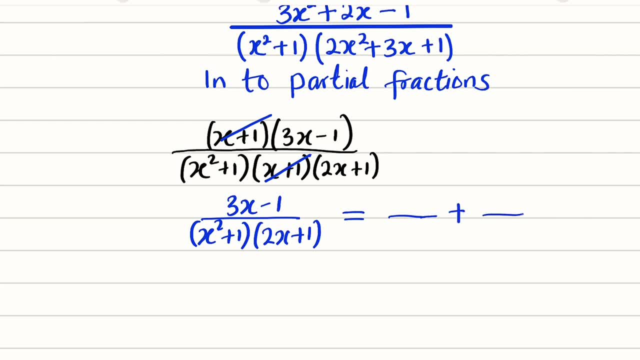 plus the second one the first fraction will contain its denominator as the first factor here 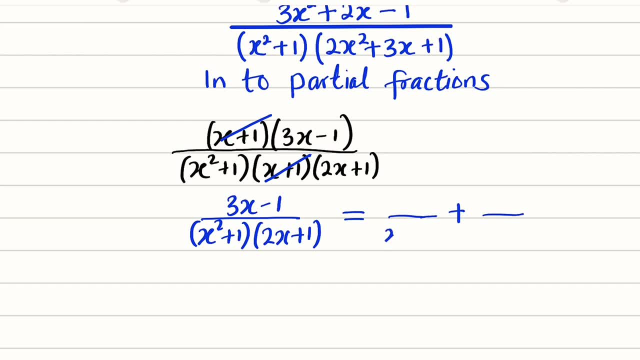 which is x squared plus 1 x squared plus 1 and the other one is 2x plus 1 2x plus 1 all right to obtain their corresponding numerators you have to also observe the nature of these two factors the numerator is 2x plus 1 the denominator is 2x plus 1 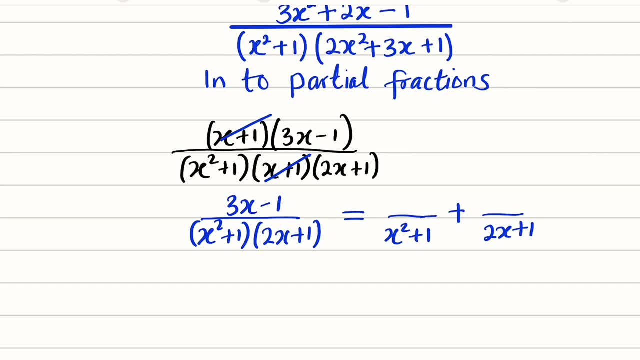 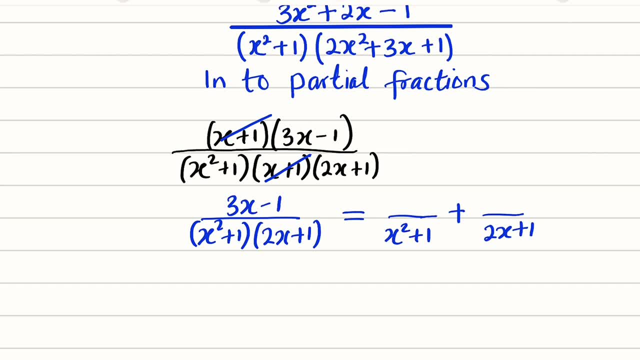 the denominator here is quadratic one degree less will be a linear so the general form is a x plus b where a and b are all constants this is linear therefore the numerator will be one degree less which is going to be just a constant and this time around we are going to use c since we have a and b we are moving now we are going to multiply 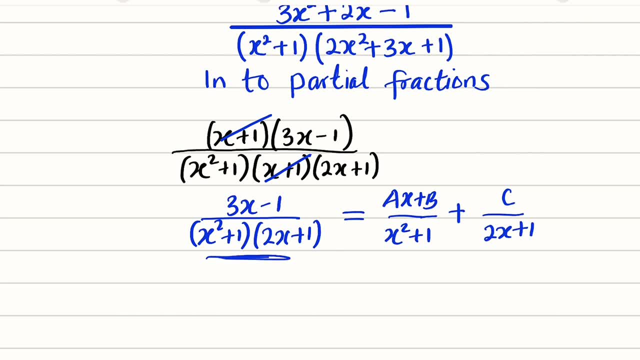 each term by these two factors in order to clear the fractions 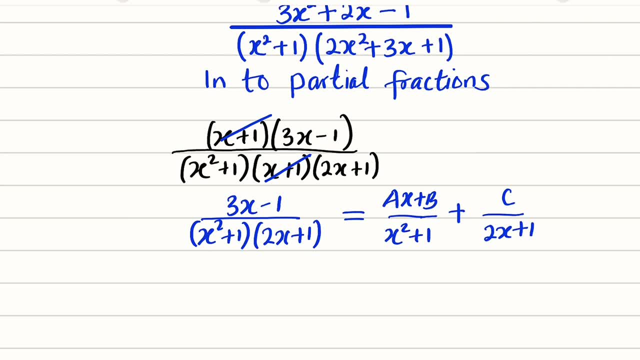 multiplying the left hand side by these two factors we will be left with only the numerator which is 3x minus 1 and to the right we have this multiplied by these two factors 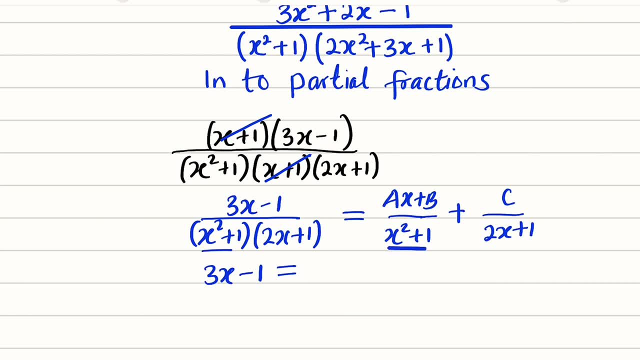 x squared plus 1 will cancel x squared plus 1 leaving only 2x plus 1 multiplied by a x plus b so, we have ax plus b multiplied by two x plus one then we add take this multiplied by these two factors 2x plus 1 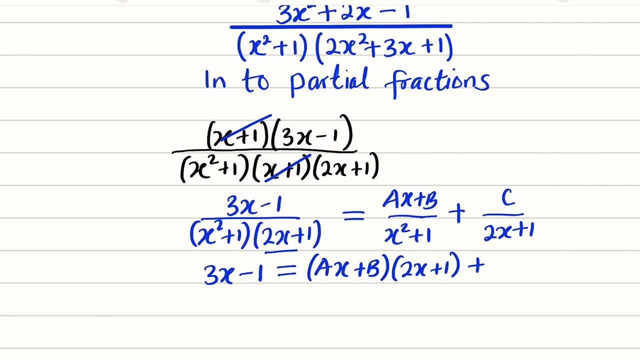 cancel 2x plus 1 leaving x squared plus 1 multiplied by c so we have c multiplied by x squared plus 1. now we are going to expand these brackets 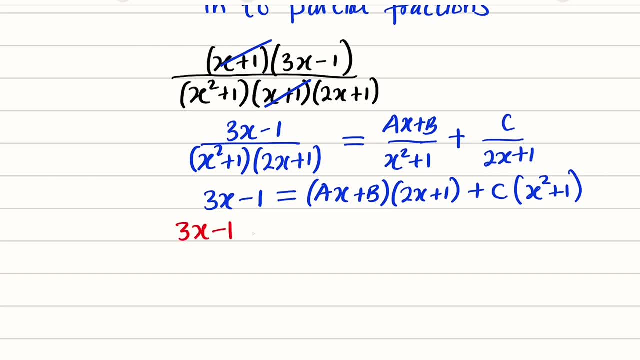 to the left we have 3x minus 1 and to the right we have ax multiplied by 2x will be equal to 2a x squared 2 a x squared take that again multiply by 1 you have a x 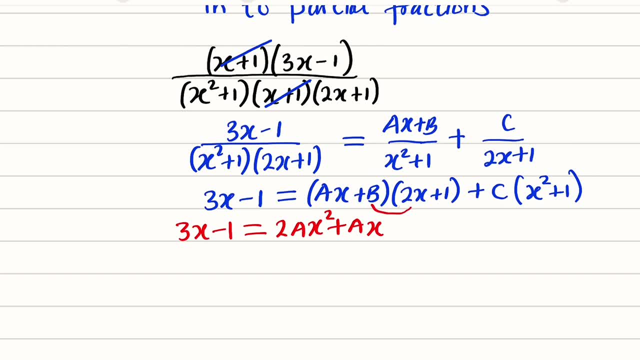 then take the second term b multiplied by 2x will be 2 b x 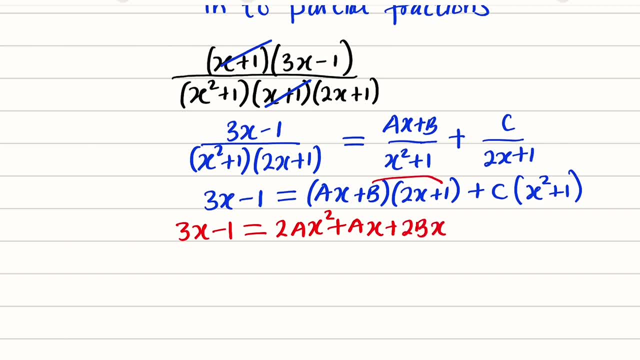 2 b x take b again multiply by 1 you have just b then the last one c multiplied by x squared will be c x squared then c multiplied by 1 is just c 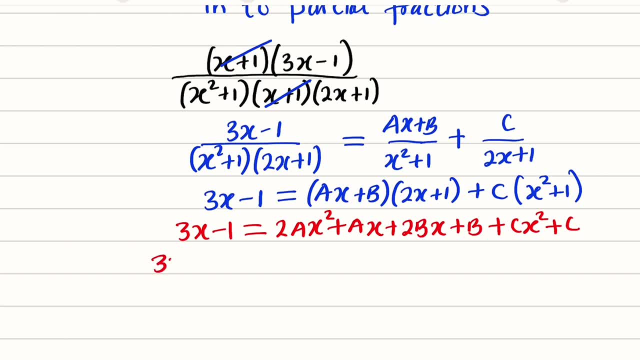 all right we are moving to the left we have 3x minus 1 and to the right we have let us bring those with x squared together we have one here and we have the other one here and we can write them as 2a then plus c so that we factor out the x squared then let us bring those with only x one here the other one is here we have a plus 2b a plus 2b all multiplied by x we just fucked out x then lastly we have our constants b and c b plus c now we are going to solve this equation by relating the coefficients 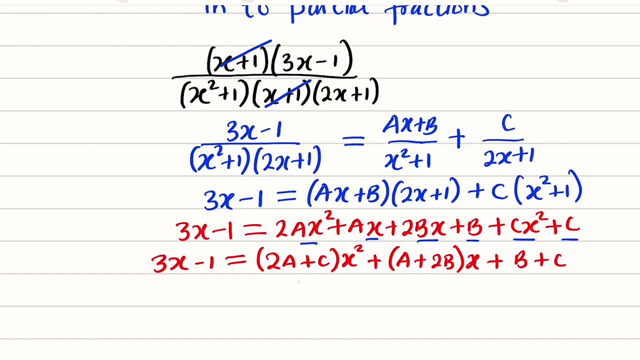 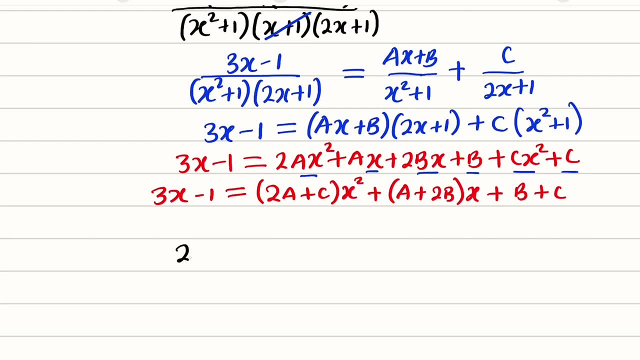 let me start with x squared the coefficient of x squared to the right is 2a plus c so our first equation is 2a plus c and what is the coefficient of x squared to the left nothing because we do not have any x squared to the left so this is equal to 0 our first equation the coefficient of x to the right is a plus 2b we have a plus 2b equals the coefficient of x to the left which is 3 here this is our second equation now let us form the last one using constants b plus c 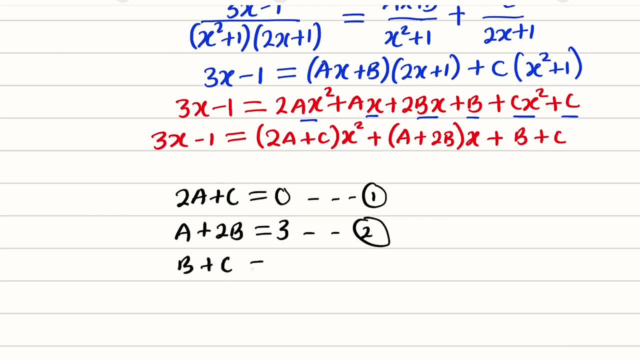 b plus c equals the constant to the left is negative 1 and this is our third equation 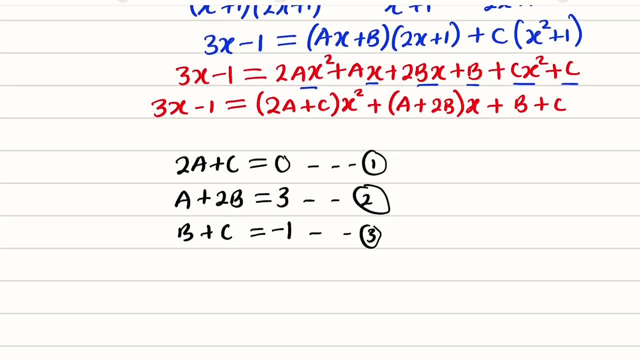 now let me use this first equation to make a the subject from equation one we have 2a 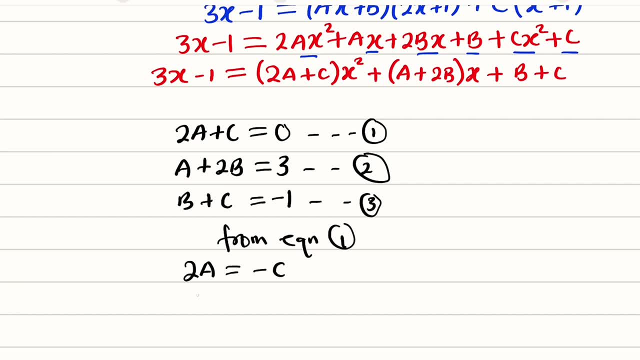 equals negative c if c crosses over and a will be equal to negative c divided by 2 and i can call this one equation number 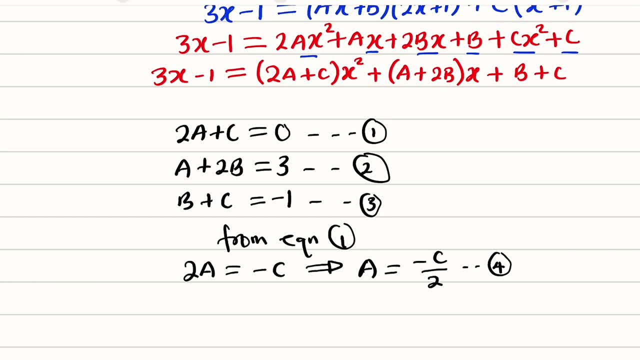 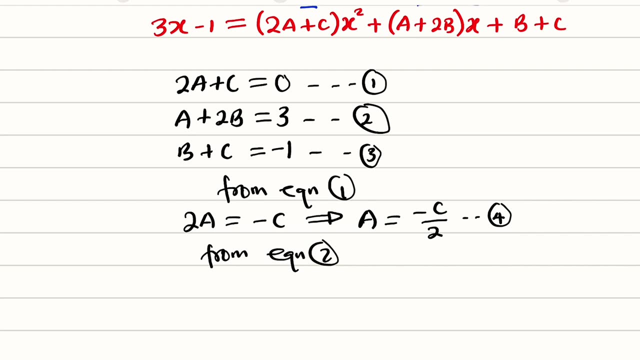 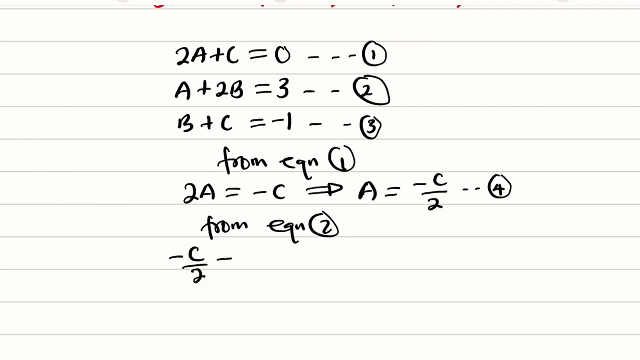 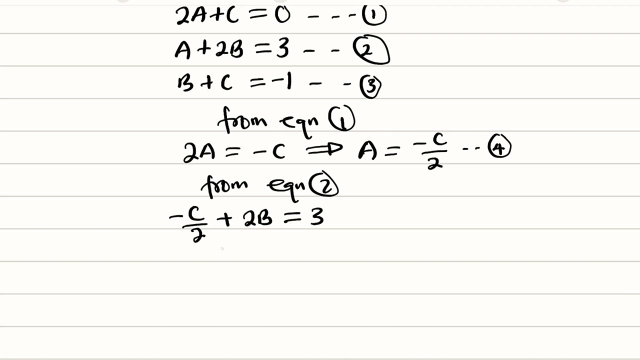 4. now we can plug equation 4 into equation 2 because we have a here and a is equal to negative c divided by 2. so from equation 2 we can write negative c divided by 2 and a plus the second term which is 2b and to the right we have 3 we can multiply each time by 2 to clear the fraction negative c divided by 2 multiplied by 2 will be negative c plus 2b multiplied by 2 is 4b To the right, 3 multiplied by 2 is equal to 6. 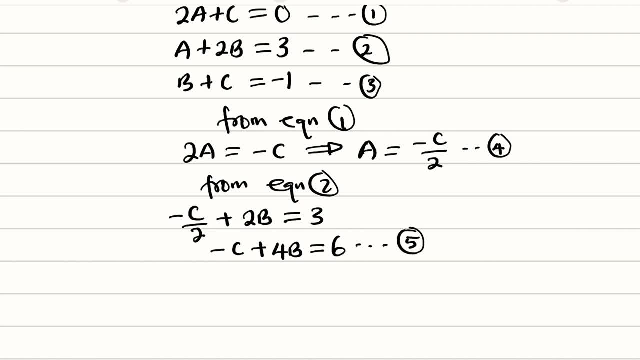 Now this is another equation we form by substitution. Now we can bring equation 3, join it to equation 5, solve them simultaneously. 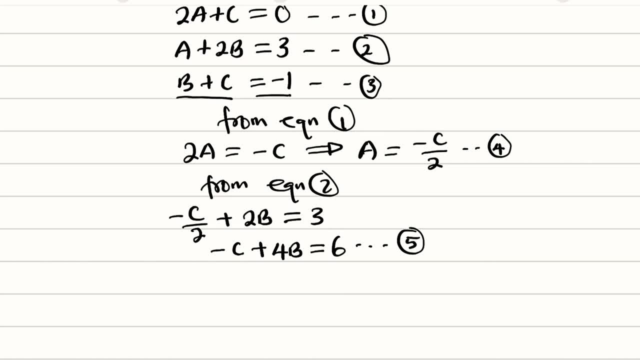 We have b plus c equal to negative 1. But I can write it as c plus b commutative. It's all the same. So, c plus b equals negative 1. 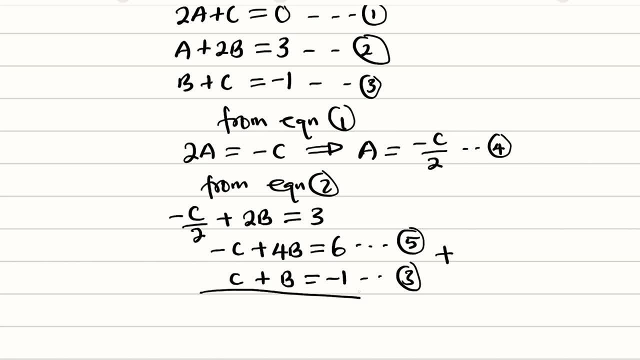 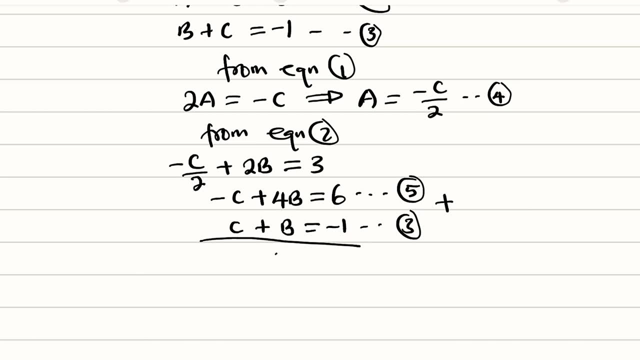 We want to add them together to eliminate c. Negative c plus c is 0. 4b plus b is 5b. 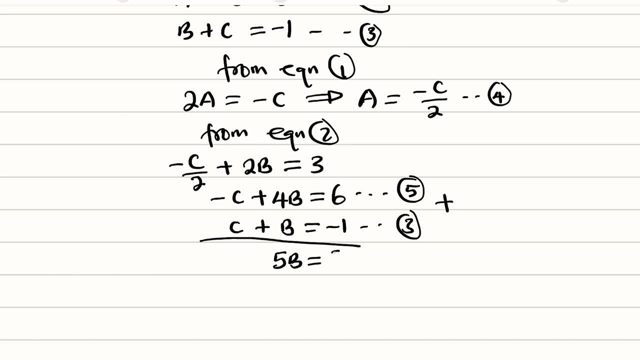 To the right, we have 6 plus negative 1, which is 5. 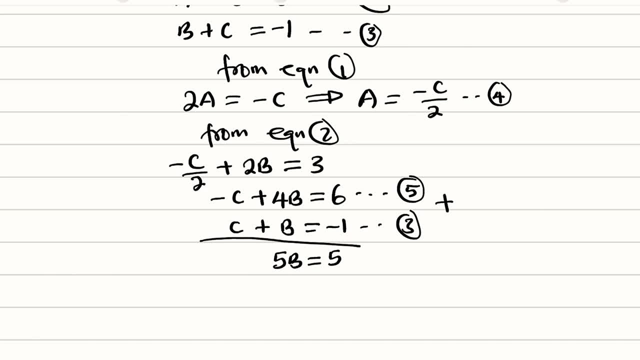 We are looking for b. We can divide both sides by 5. Therefore, b equals 1. We have just obtained one of the values we are looking for. 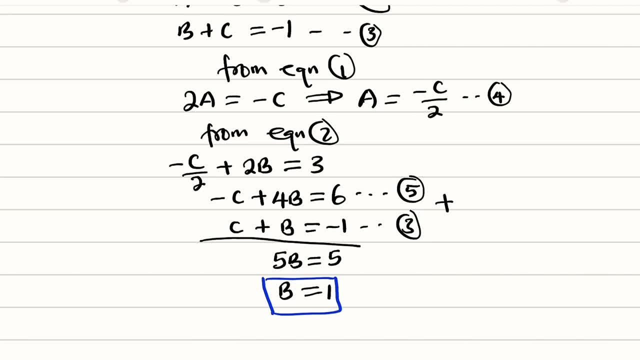 Now we can plug it back into this equation number 3 to obtain the value of c. From equation 3, 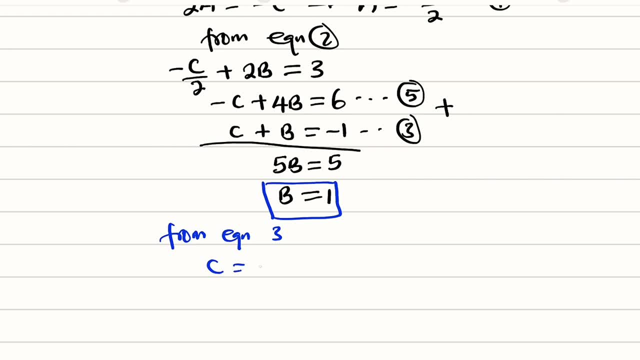 you can see that c is equal to negative 1, negative b if b crosses. But b is 1, so we have c equals negative 1, negative 1. This implies that c is equal to negative 2. Another value of 10. 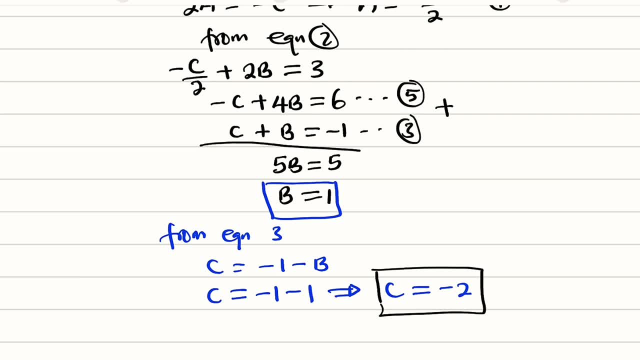 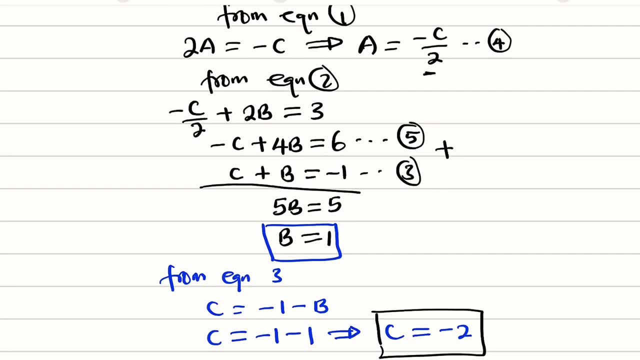 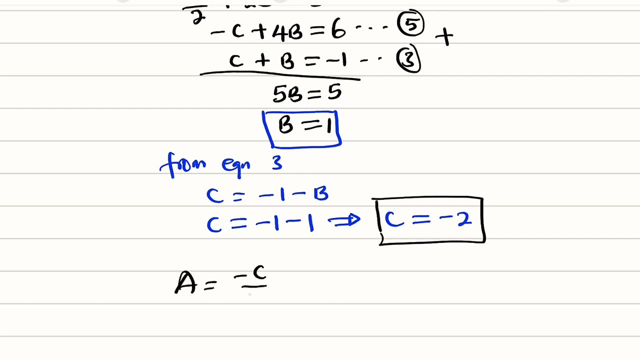 And the last one we want to find is the value of a, which is negative c divided by 2. You can see it right here. So, a is equal to negative c divided by 2. But c is negative 2, so a will be equal to negative negative 2 divided by 2. And finally, a is equal to 1. This is another value, and this is the last one. 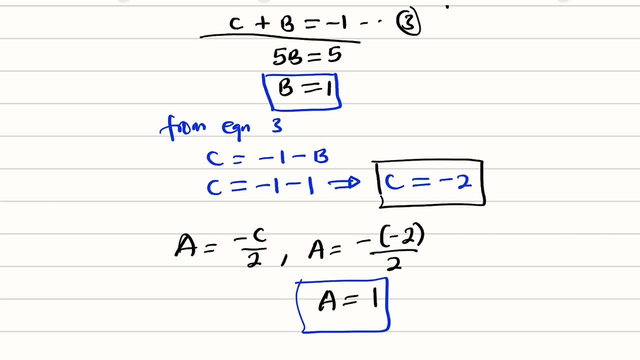 Now, what do we need to do next is to substitute a, b, c in this fraction. You can see them right here. 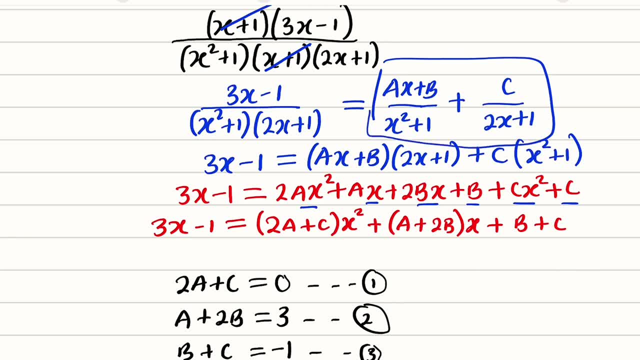 We are going to substitute the values of a, b, and c there to obtain our partial fractions. So, now let me copy that. 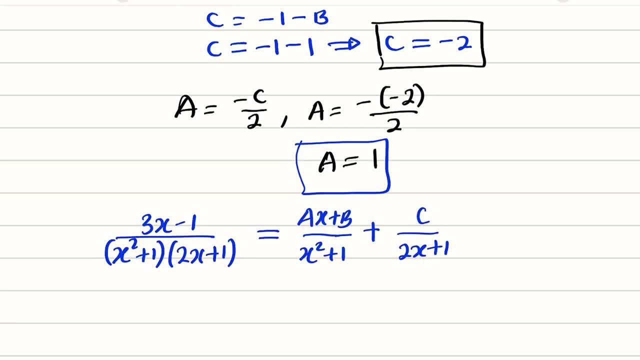 So, I have just copied the equation here. We are going to substitute for a, b, and c. 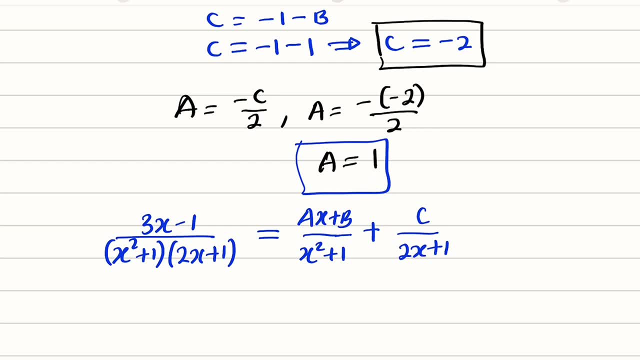 For a, we can see that it is equal to 1. So, we have 1 multiplied by x, which is the same thing as x, plus 1. b is equal to 1. You can see it right here. So, plus 1. 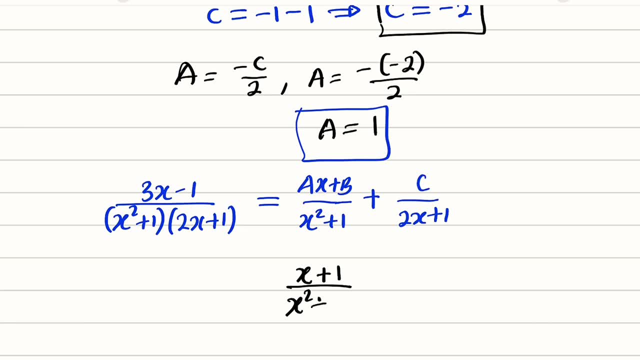 Divide by x squared plus 1. 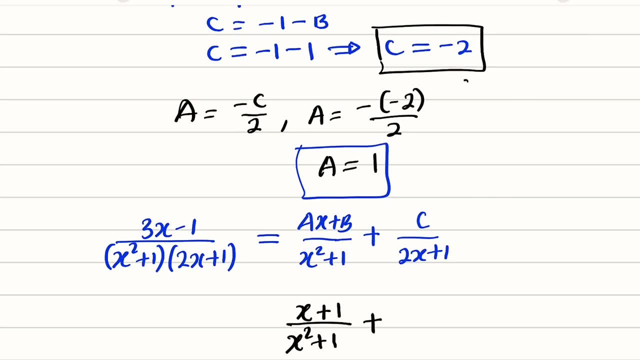 Then, plus c is negative 2. You can see it right here. So, this is negative instead of positive. 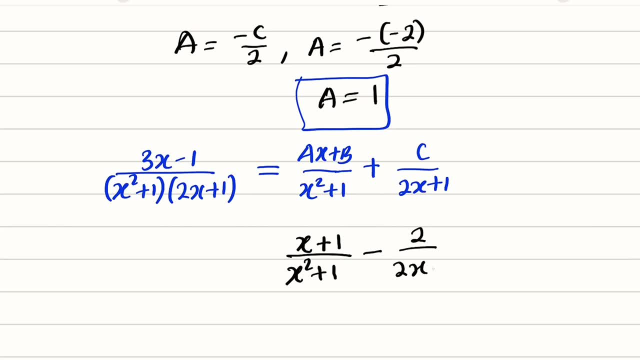 2 divided by 2x plus 1. 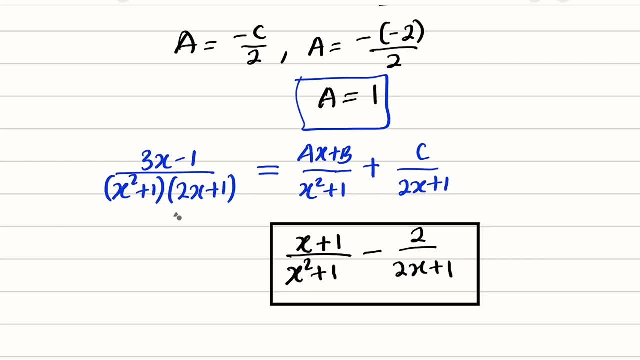 And this is the... This is the partial fraction of this compound fraction.